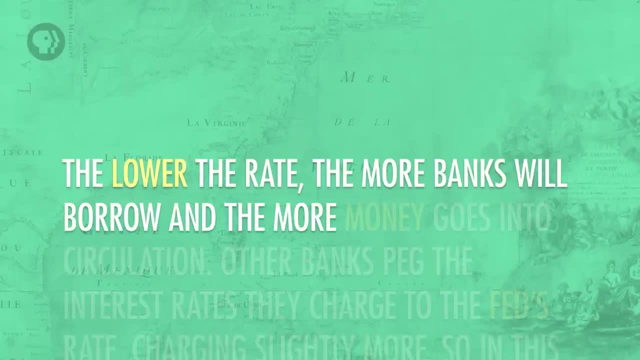 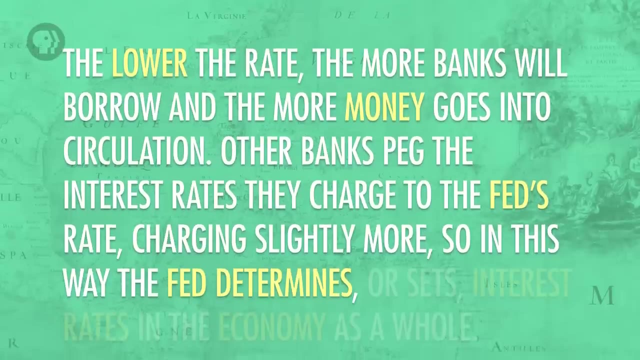 mostly how much money banks will borrow. The lower the rate, the more banks will borrow and the more money goes into circulation. Other banks peg the interest rates they charge to the Fed's rate charging slightly more. So in this way the Fed determines or sets. 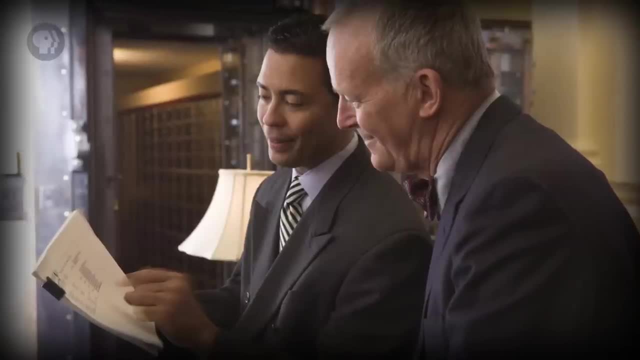 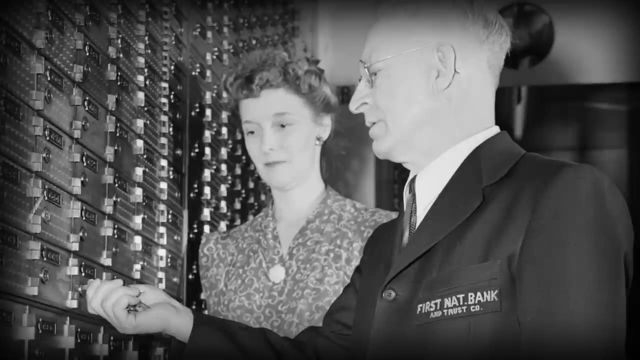 interest rates in the economy as a whole. The Fed also creates regulations that control how much money circulates in the economy. One of these is the bank reserve requirement, or the amount of money in cash that a bank has to have on hand. Now, the amount of money. that a bank holds in reserve is only a fraction of the total amount of money held in deposit at the bank. That's why it's called fractional reserve banking. But the reserve requirement is there so that you don't get catastrophic bank runs like we saw during the Great Depression when 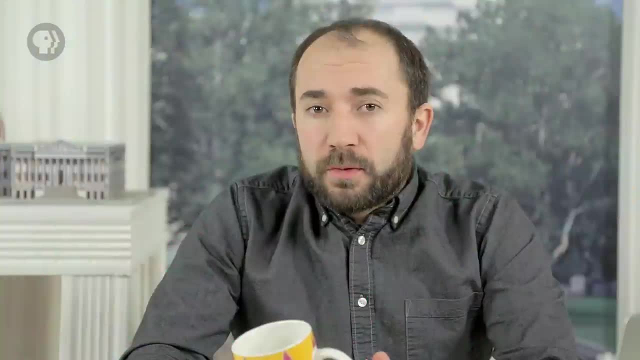 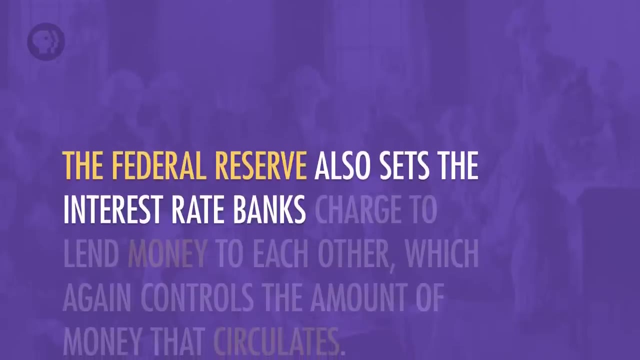 so many frightened depositors took their money out of the banks that the banks failed. Raising the reserve requirement reduces the amount of money in circulation and lowering it pumps more money into the economy. The Federal Reserve also sets the interest rate banks charge to. 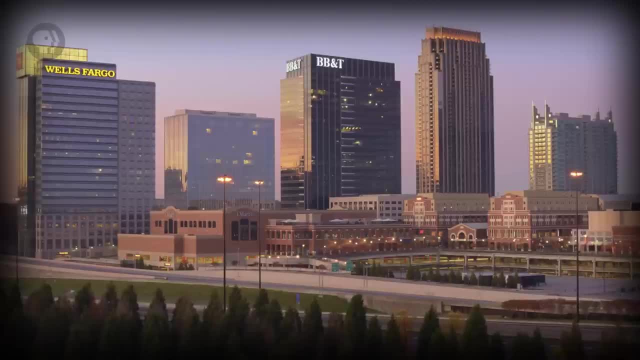 lend money to each other, which again controls the amount of money that circulates. If banks are charging each other a lot of money to borrow, they won't borrow as much and they won't lend as much to firms and individuals, and there will be less money in the economy. 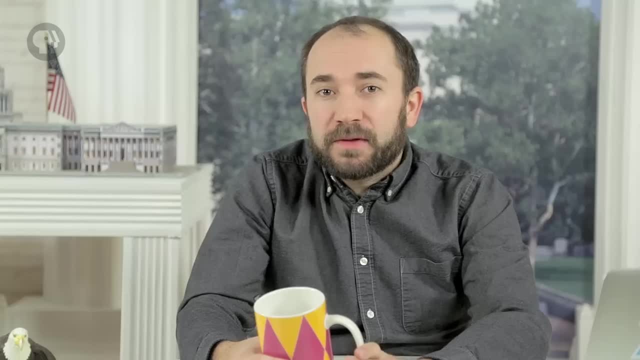 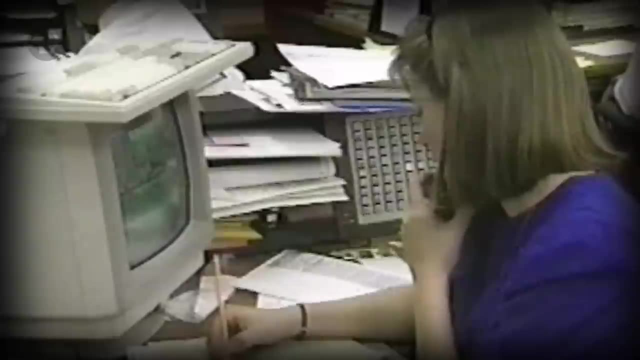 as a whole. There's at least one more important way that the Fed influences the money supply in the US, and that's through open market operations. This is a fancy way to say that the Fed buys and sells government debt in the form of treasury bills or government bonds. When the Fed sells, 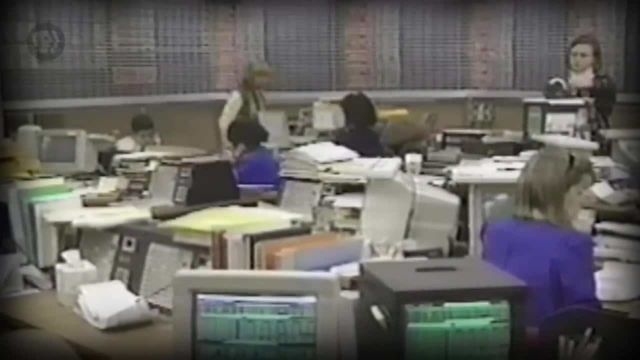 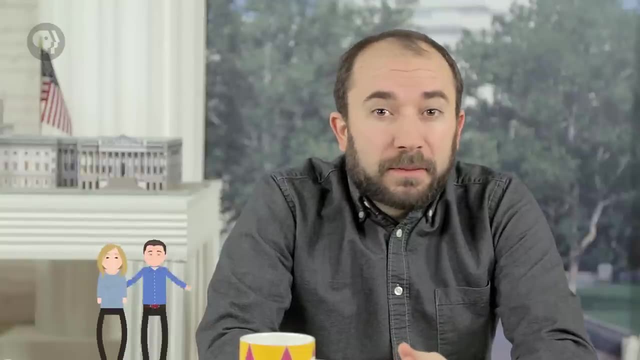 bonds, it takes money out of the economy and when it buys them, more money goes into the economy. This is the idea behind what is known as quantitative easing, which is really complicated. To be honest, I'm not crazy about wading into economics here, and 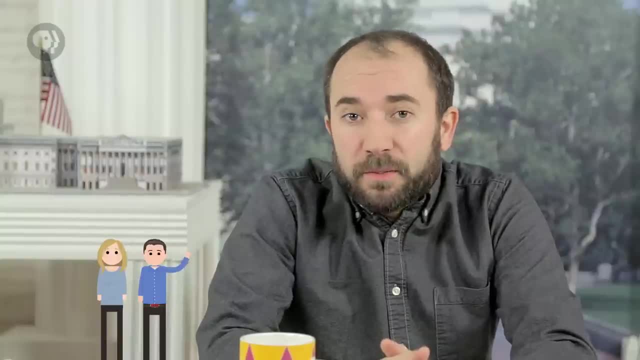 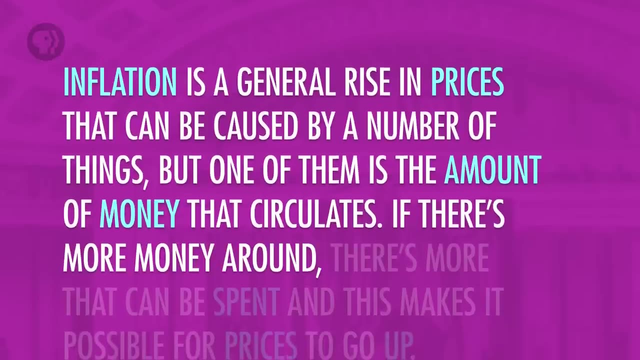 thankfully, there's a whole other series to do that, but I have to mention inflation at this point. Inflation is a general rise in prices. that can be caused by a number of things, but one of them is the amount of money that circulates, If there's more money around. 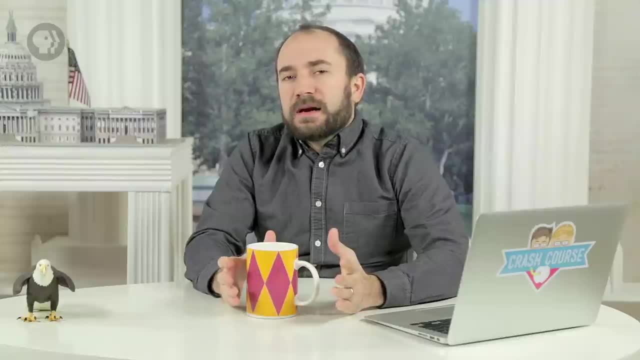 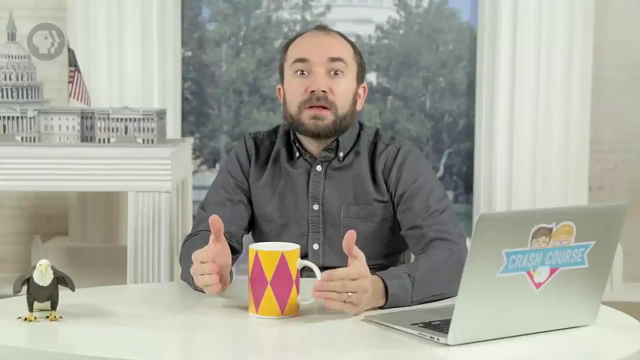 there's more that can be spent, and this makes it possible for prices to go up, But this isn't an absolute rule. As of 2016,, we've had years of basically zero interest rates, which means it's really cheap to borrow money, which means that there should be a lot of. 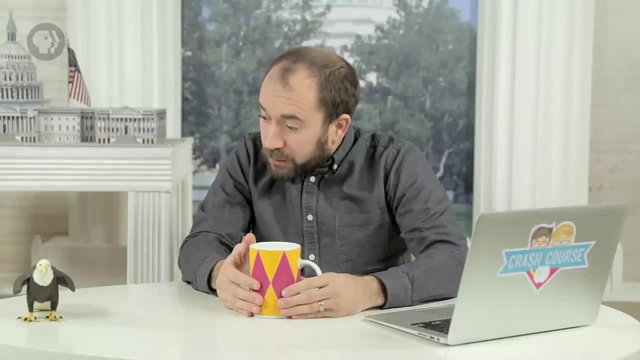 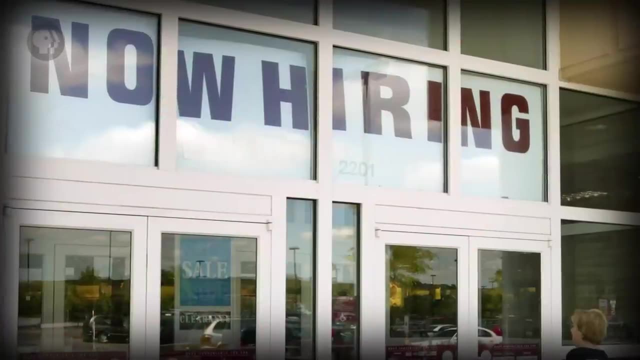 money in circulation, Yet inflation remains quite low. Hey, it's real cheap to borrow money. Can I borrow two bucks? No, He never has any money. Usually, low interest rates tend to cause inflation and reduce unemployment, and high interest rates are expected to cool down in overheating as a result of inflation In the 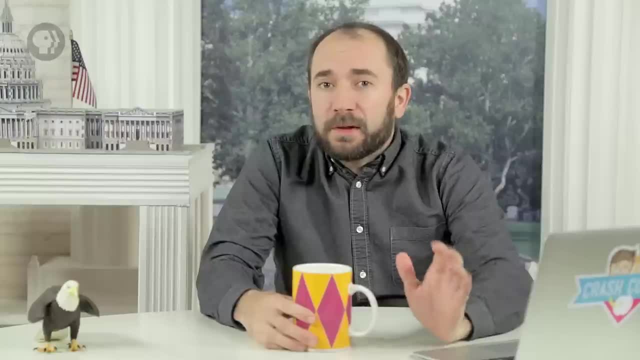 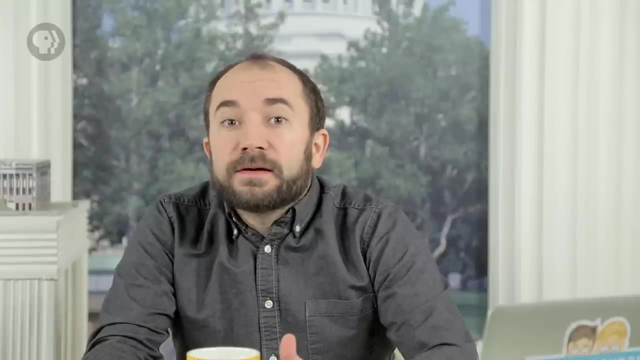 economy, But that hasn't happened much in the past few years. I'll say again: I'm glad this isn't an economics series. It's important to note here that the Federal Reserve is an independent body, meaning that its board of governors and chairperson are not elected. 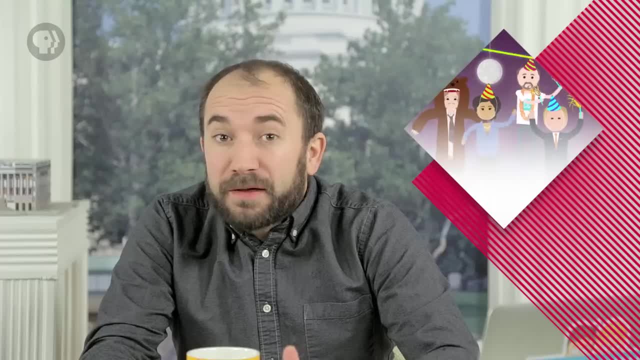 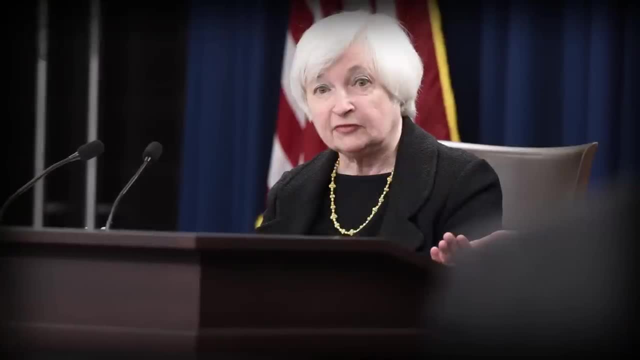 or really subject to much regulation from Congress, And they throw the best parties. That's probably why This is intentional and probably a good idea. Ideally, you want people in charge of the money supply to be able to look after broader interests than their own. 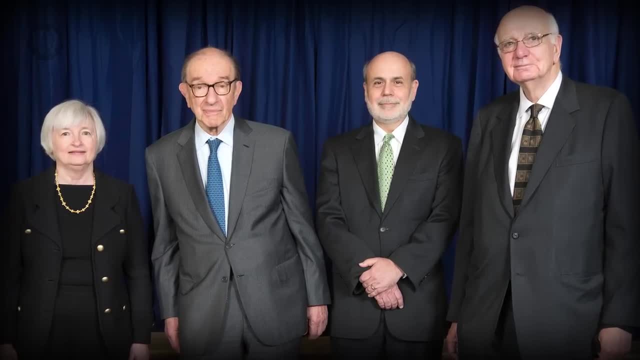 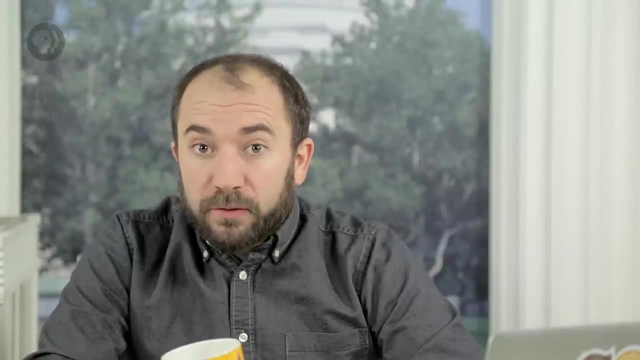 re-election, and this is why the Fed is supposed to be insulated from politics and remain independent. Okay, so that's monetary policy, which is one lever that the federal government has to use to influence the economy Increasingly. it's the only lever, because in America, 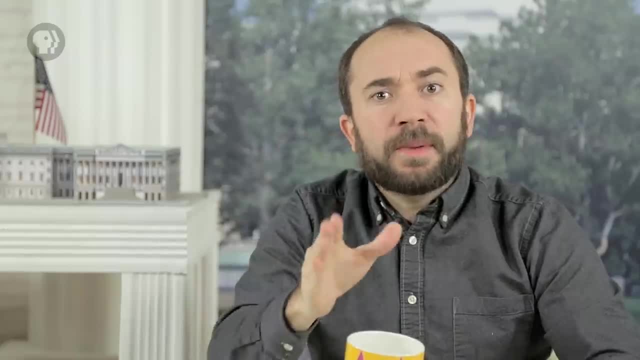 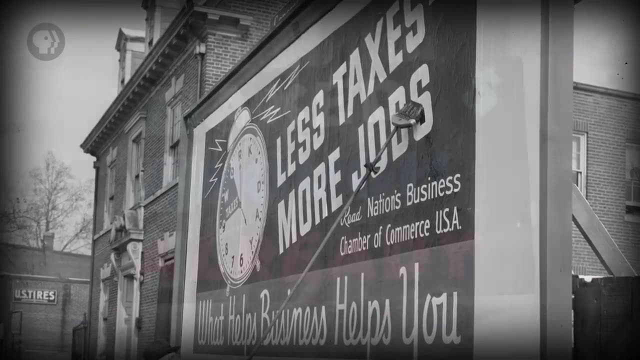 we have a hard time with fiscal policy. What's that you might be asking? Fiscal policy refers to the government's ability to raise taxes and spend the money it raises. Since I know that, by this episode, you've been paying a lot of attention to American politics, you 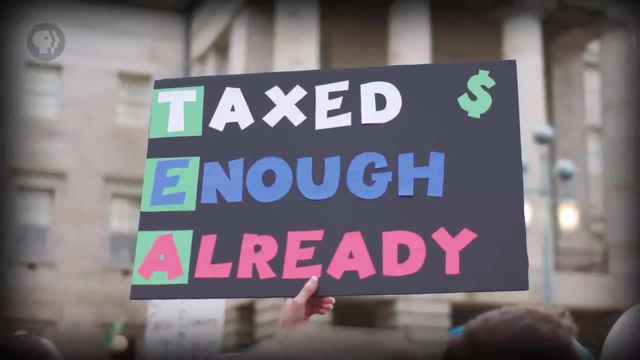 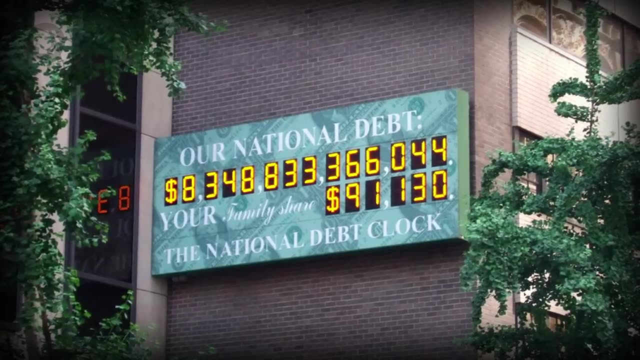 know that in the past twenty or thirty years at least, Americans have generally been reluctant to raise taxes and somewhat reluctant to have the government spend money. The difference between these two goals- spending money and not raising taxes- largely explains why we have deficits Before we get into tax policy, which I know is what you've been waiting. 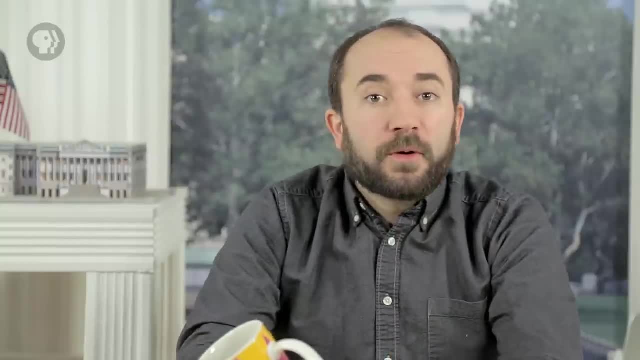 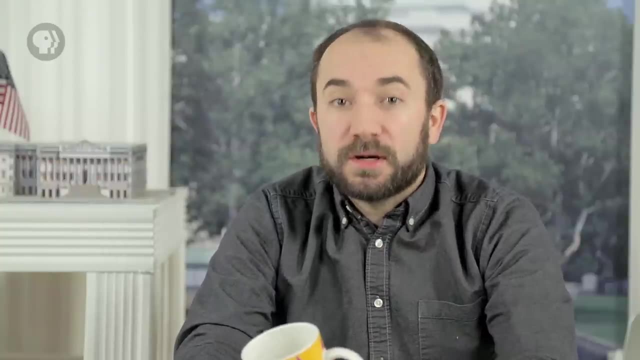 for calm down. I need to point out that the way the government can spend more money on programs than it takes in taxes is by borrowing it, which the government does by- you guessed it- selling bonds. Good thing we talked about open market operations. 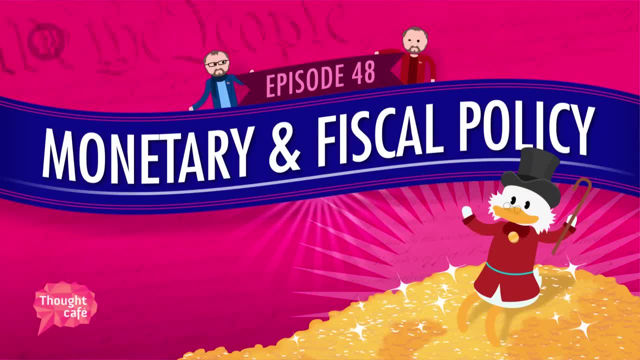 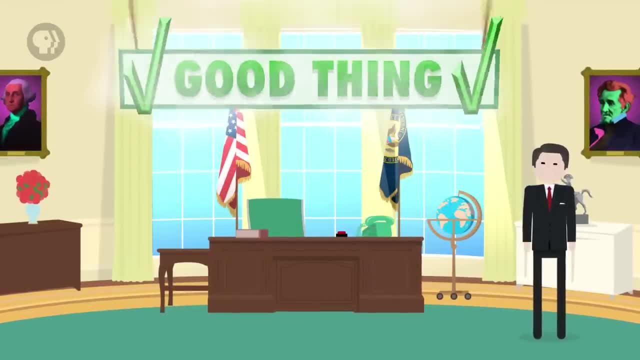 Let's tax the Thought Cafe people with a lot of work by talking about taxes and spending in the Thought Bubble. First ever since Ronald Reagan came to office, there has been a hostility towards higher taxes and government spending that is theoretically based in an idea called 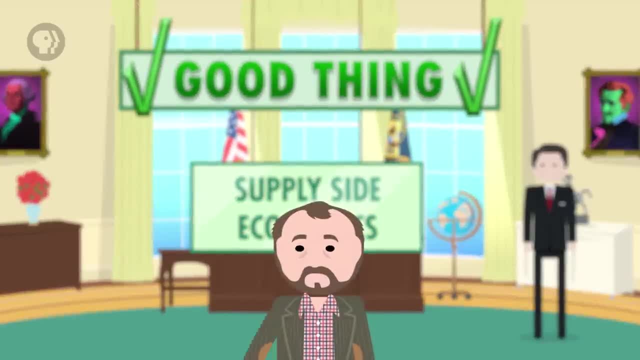 supply-side economics. I'm not going to discuss the details of the theory, or even whether it's right or wrong or somewhere in between, But the basic thrust is that the idea is based on supply-side economics. I'm not going to discuss the details of the theory, or even whether it's right or wrong or somewhere in between, but the basic thrust. 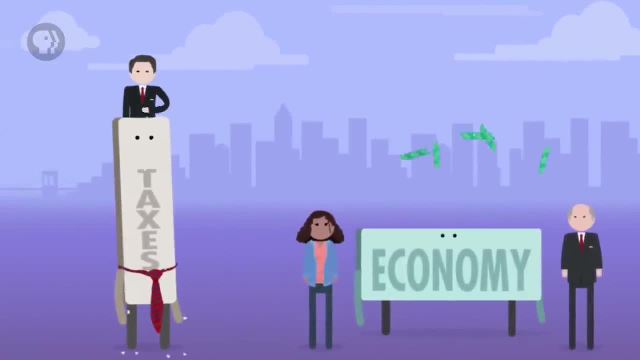 is that if you lower taxes on businesses and individuals, the individuals will be able to spend more, the businesses will be able to invest more and the economy as a whole will grow. It's a simple and politically powerful idea and has set the terms of the 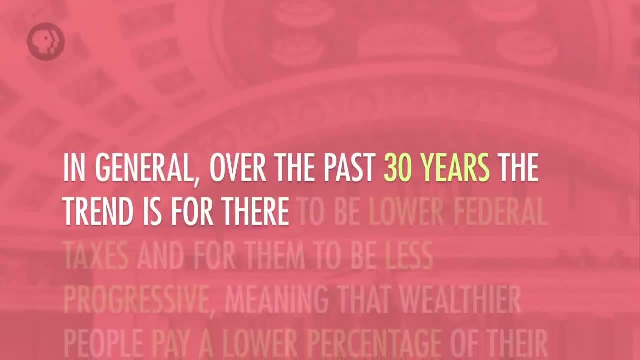 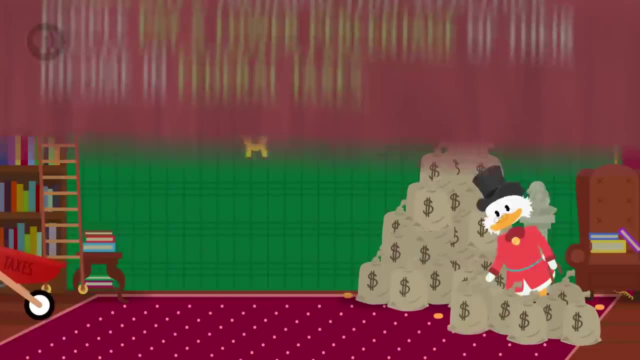 debate for a generation. In general, over the past thirty years, the trend is for there to be lower federal taxes and for them to be less progressive, meaning that wealthier people pay a lower percentage of their income in federal taxes. The wealthy still pay the. largest share of federal taxes overall, so it's not completely accurate to say they aren't paying, though. Since Reagan, and especially during the presidency of George W Bush, income income tax rates on the highest earners have fallen, as have taxes on estates, although they did go up again. 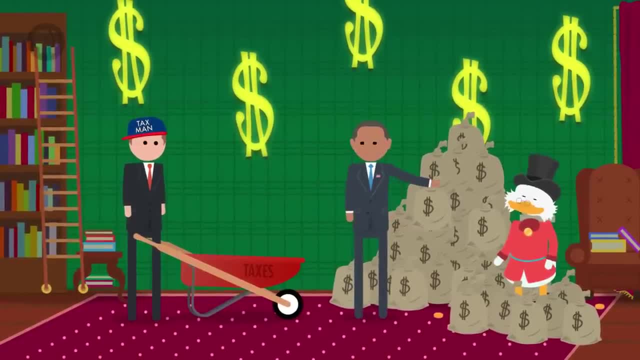 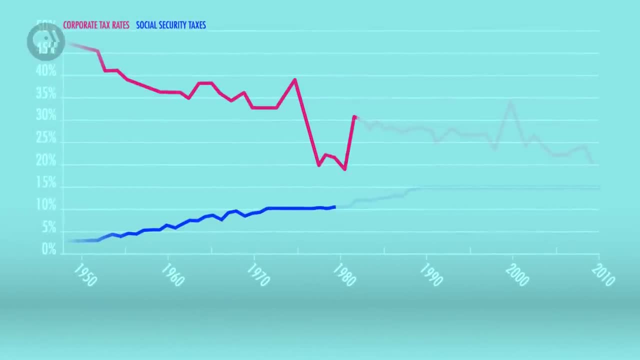 and on capital gains and dividends. President Obama did raise taxes, but primarily on people earning above $450,000 a year. Corporate tax rates have also declined and Social Security taxes have gone up, which is important because this is the federal tax that most of us are most likely to pay. 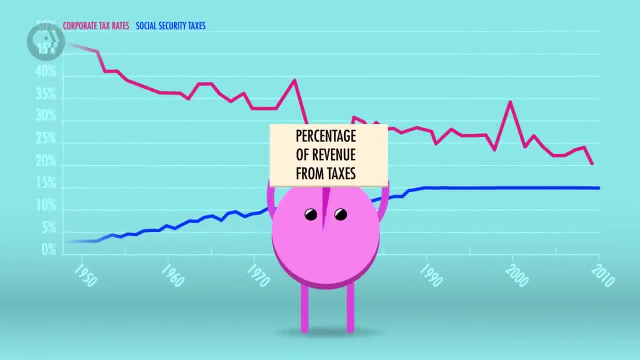 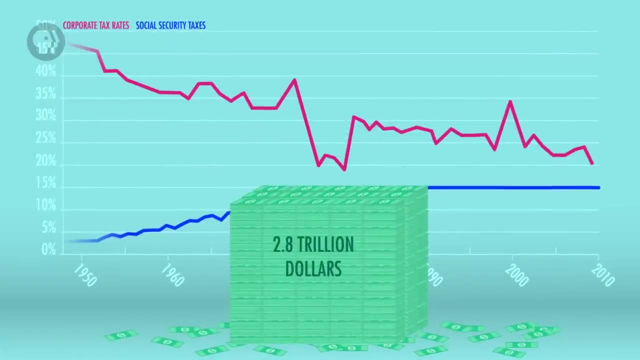 Overall, the percentage of revenue that the federal government receives from taxes has held pretty steady, at between 43% and 50%. If you're interested in the numbers for 2013,, the government received almost $2.8 trillion in tax revenues. 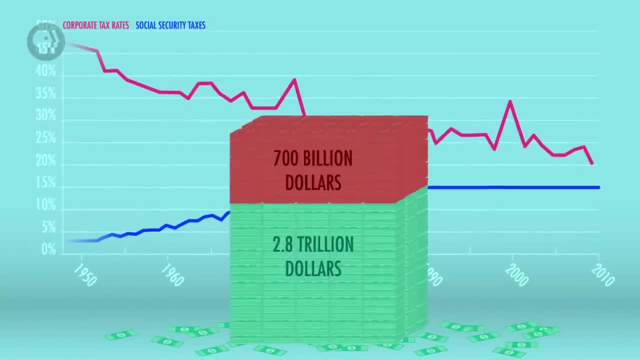 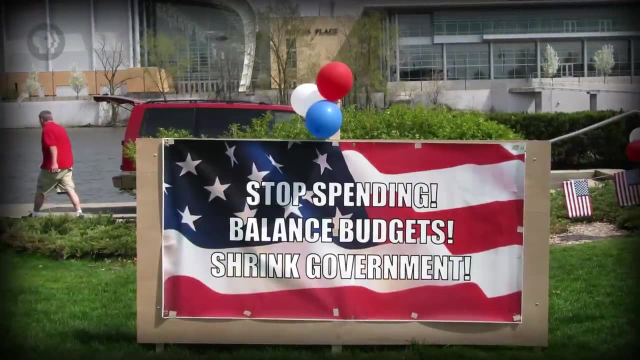 and it spent $3.5 trillion, which math tells us means a deficit of around $700 billion. Thanks, Thought Bubble. When people say that they need to cut spending and balance the budget, this is what they're talking about. but it's not quite as simple as just spending less, because there are some places where the government can't cut spending, even if they want to. 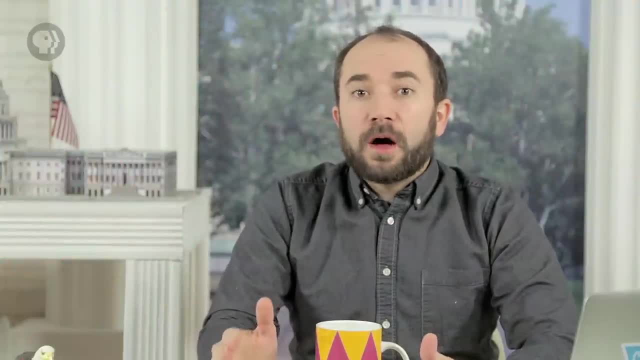 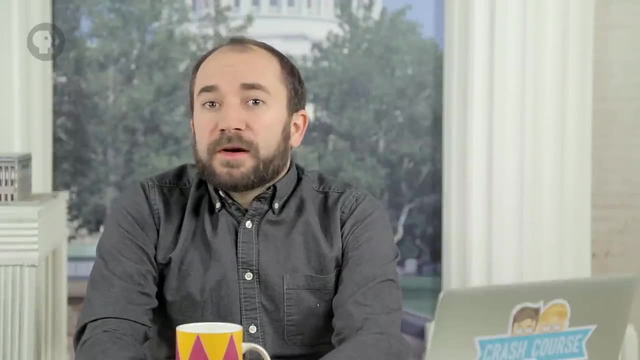 There are certain items in the federal budget that must be spent because they are written into law by Congress. These are called uncontrollables or mandatory spending. One uncontrollable that relates to monetary policy is the tax rate. Monetary policy is interest payments on federal debt. 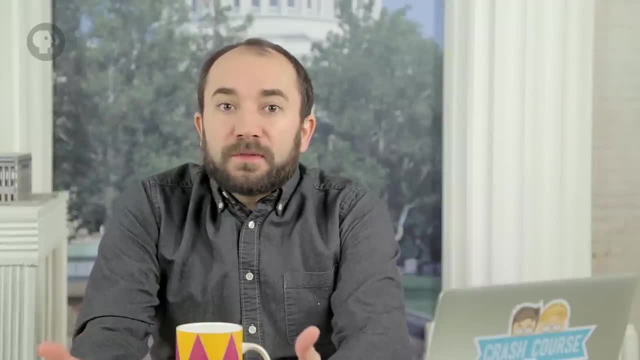 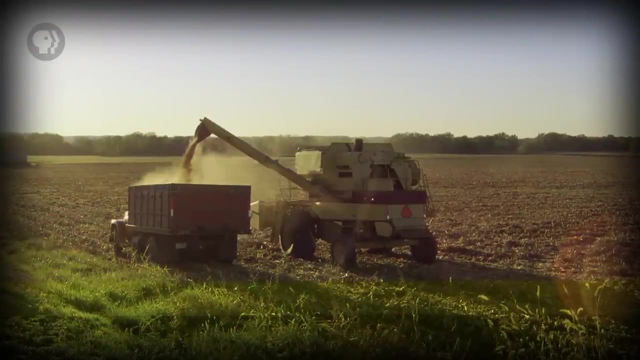 The government can't not pay its interest, Otherwise no one would lend us money. That's just how lending works, or it's supposed to work. Farm price supports subsidies are also counted as uncontrollables, and they are important, but not nearly as important as the two big-ticket mandatory spending items. 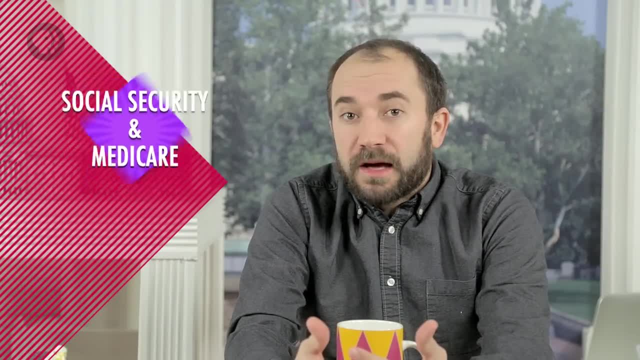 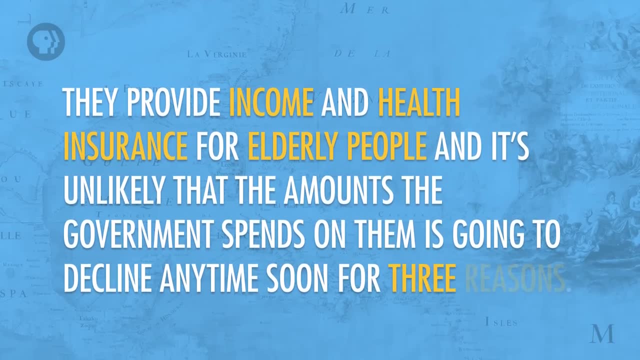 These are Social Security and Medicare, and they're paid for with dedicated federal taxes. They provide income and health insurance for elderly people, and it's unlikely that the amounts the government spends on them is going to decline any time soon, for three reasons. First is that the population is aging. 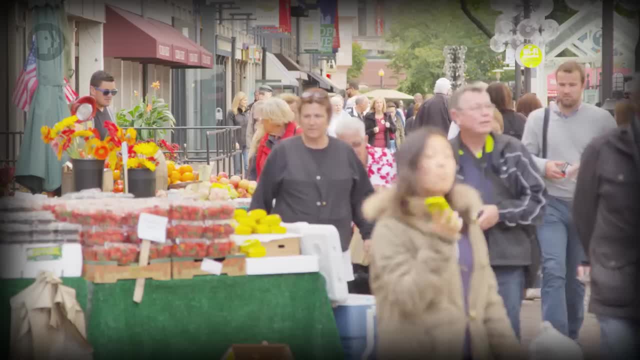 meaning that the percentage of income that the government spends on them is going to decline any time soon, for three reasons. The percentage of older Americans is rising in proportion to younger Americans. This means that more people will be receiving Social Security payments, which leads us to the second reason: they are unlikely to go down. 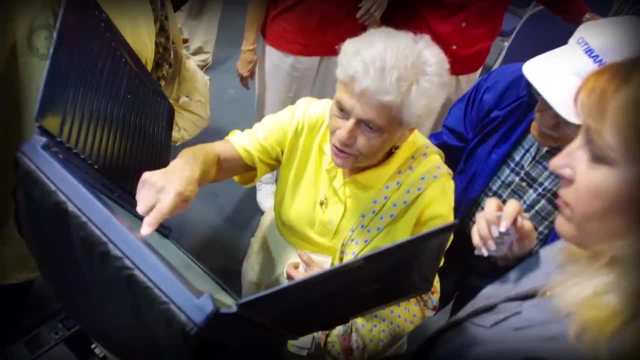 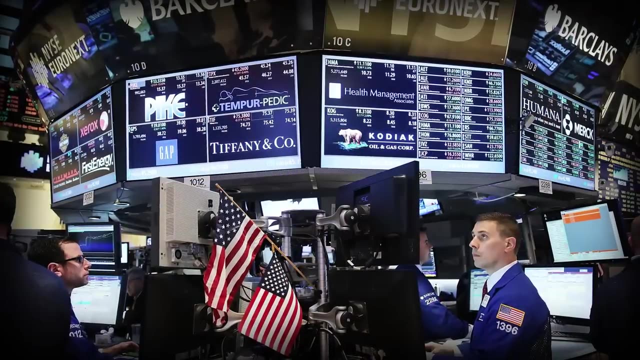 People like them. The third reason is more political. Older people tend to vote more regularly, so a politician who wants to keep their job is unlikely to vote for cuts in Social Security or Medicare. So here's the thing about the Federal Reserve and economics. 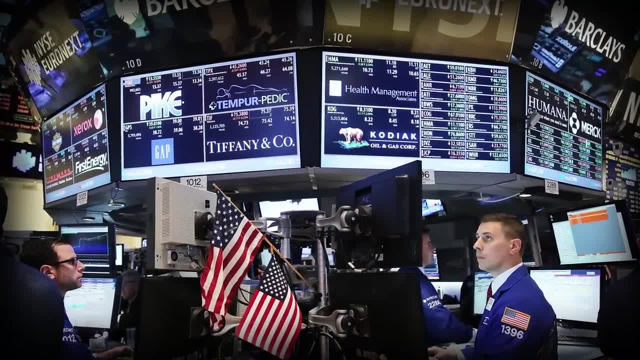 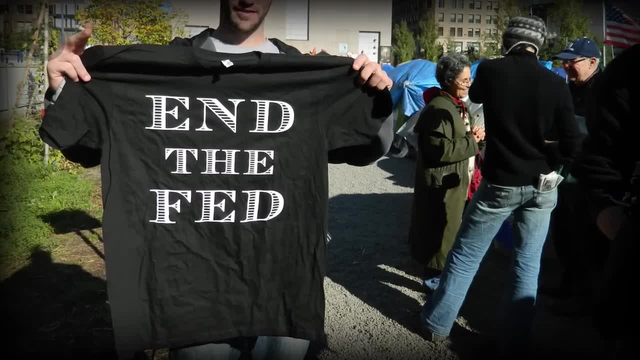 The American economy is really huge and really complicated, and it has some issues that need addressing. Whether you care a lot about budget deficits or don't think they're a big deal will depend a lot on your feelings about economics in general, But there are a couple things to keep in mind. 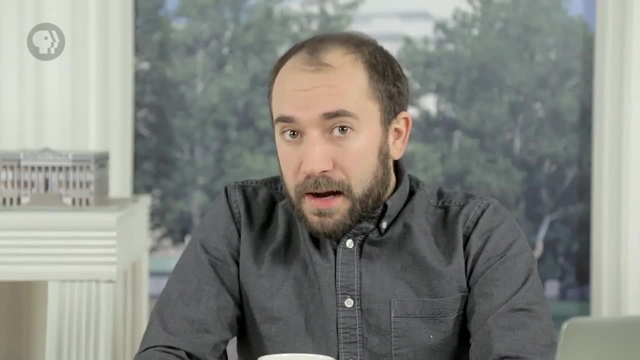 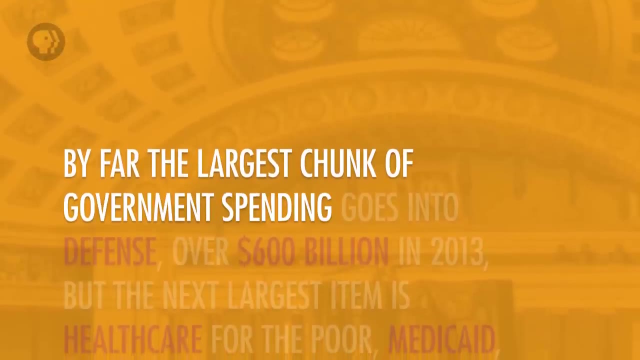 First, there's only a limited range of programs on which the government can choose to spend or not spend. These are called discretionary spending, and when people call for cuts in government spending, this is what they mean. By far the largest chunk of government spending goes into defense. 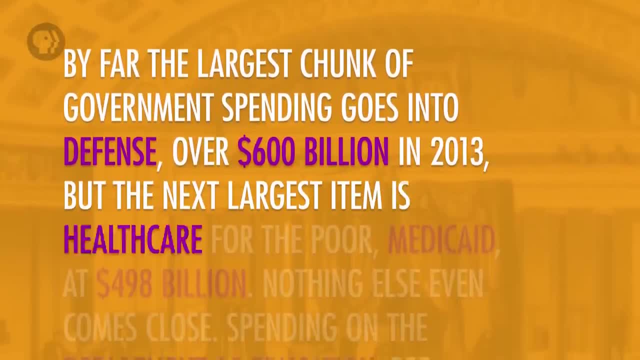 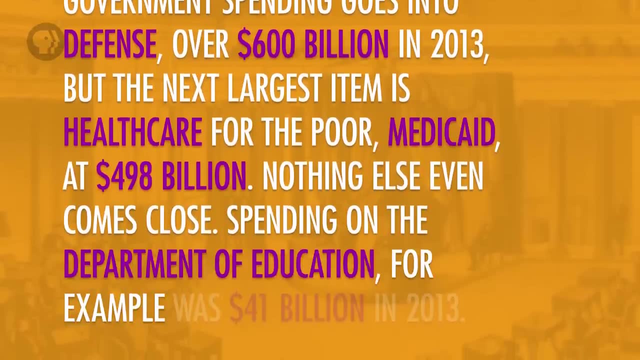 over $600 billion in 2013.. But the next largest item is health care for the poor, Medicaid at $498 billion. Nothing else even comes close. Spending on the Department of Education, for example, was $41 billion in 2013..